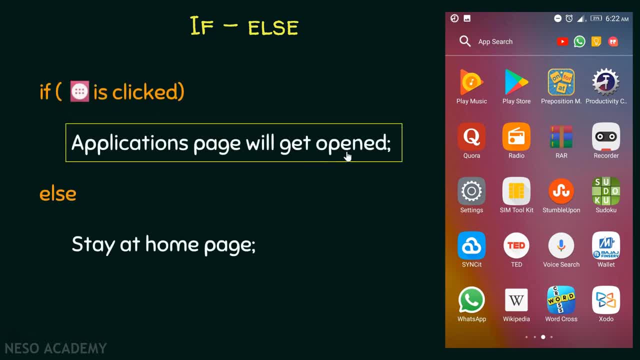 If this button is clicked, then the application's page will get opened up, Right Else, you will simply stay at home page, Isn't that so? Because opening up of this application's page is actually dependent on this button clicking. therefore, we can. 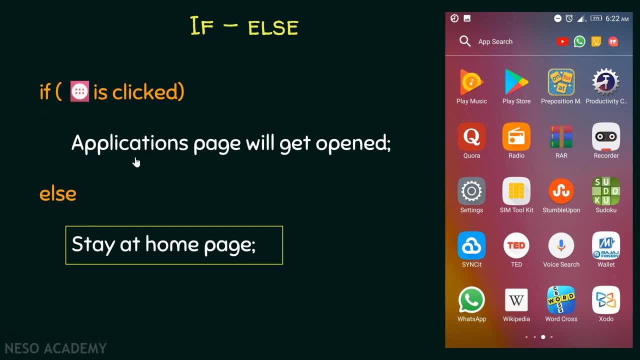 actually use if-else construct here. Whenever something is dependent on something, then we can use if-else construct. Now let's try to understand what is nested-if and when to use nested-if. Again, let's consider our real world example, that is, android operating system interface. 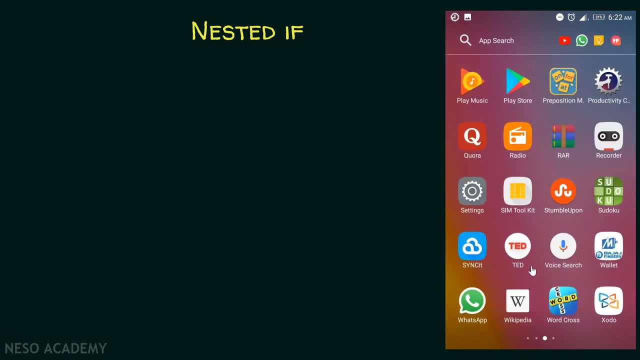 When you click on this button, then the application's page will get opened up. And suppose I want to open up an application like, suppose, play store, Then I need to click on this button, Then the play store will get opened up. Now you might ask me this question: 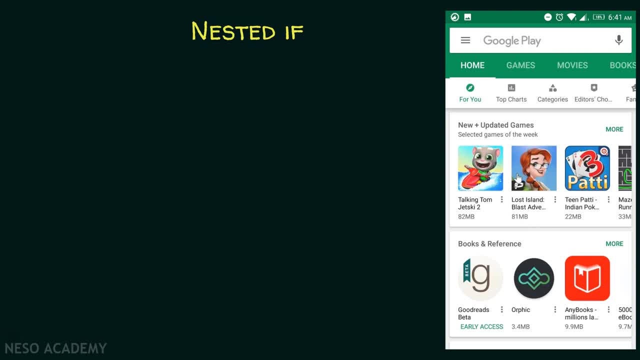 how we can relate this concept to nested-if and why I am telling all this Simple. If you click on this button, that is, this round button, then the application's page will get opened up, Right? You know that already. After that, if you click on this button, 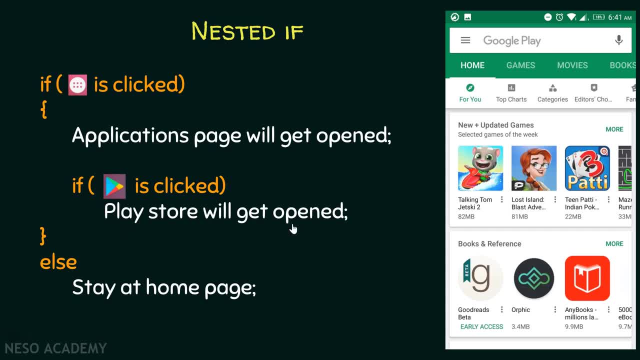 this play store button, then the play store will get opened up. That means, if you really want to open up the play store, you first have to click on this button. then only you would be able to click on this button, Isn't that so? 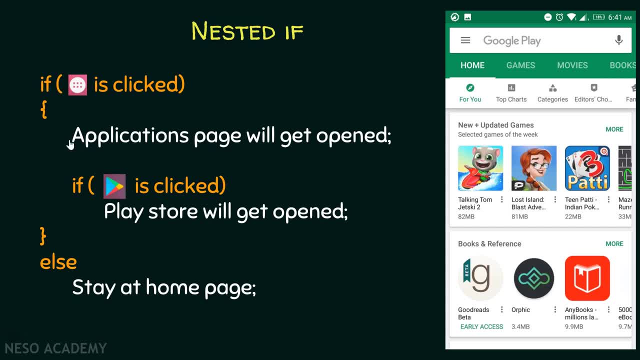 This whole if-construct is dependent on this if-construct. Therefore it has to be put inside of this if-construct. Whenever there is an if-construct inside another if-construct, then it is called nested-if construct. Please remember this point. 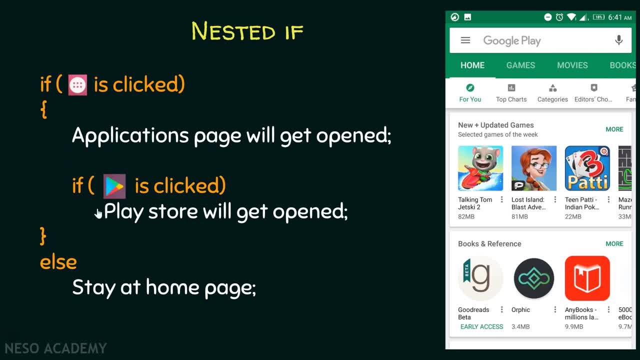 We cannot put this outside of this if-construct, because the only way you would be able to access this play store button is by clicking on this button. If you won't click on this button, you will simply stay at home page, Right, So we can easily see how. 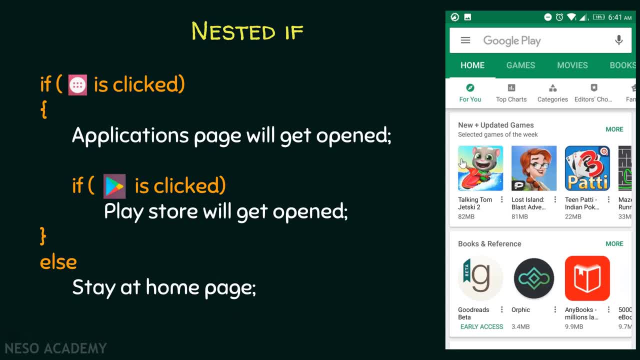 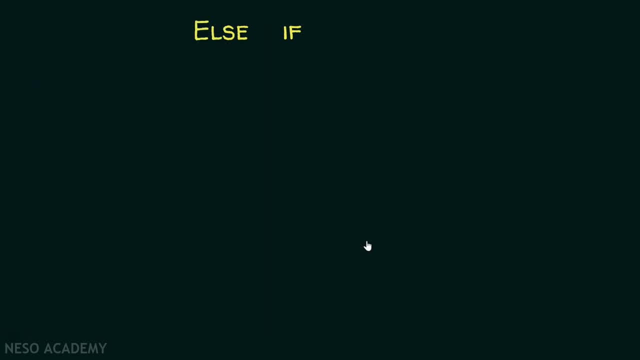 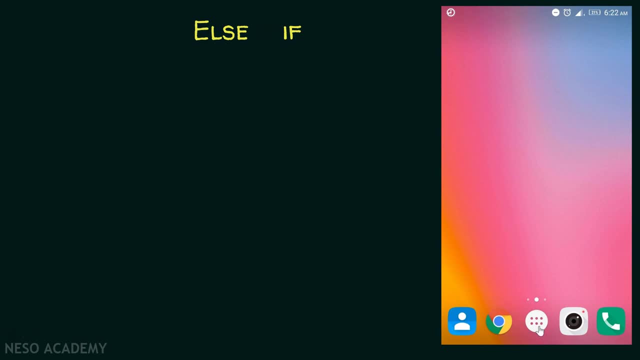 this nested-if construct is useful in our real world application like android operating system. Now let's consider why to use lsif and when to use lsif. Again, we will consider our real world example, that is, android operating system. Suppose android operating system. 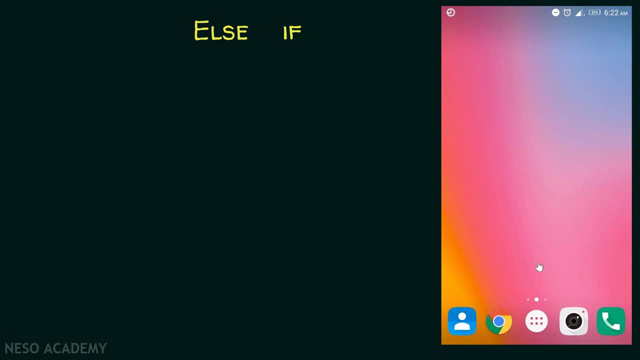 provides you the facility to add shortcuts in your home screen itself. As you can see here, these are the shortcuts: Right, This is camera application button, this is contacts application button and this is chrome application button. Now, instead of clicking this button, 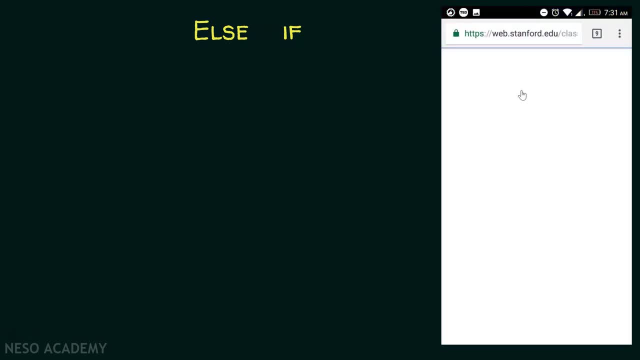 if we simply click on this button, then the chrome application will open up. Right, How I can relate this concept to lsif. Simple: If this round button is clicked, then definitely applications page will get opened up. But if we directly, 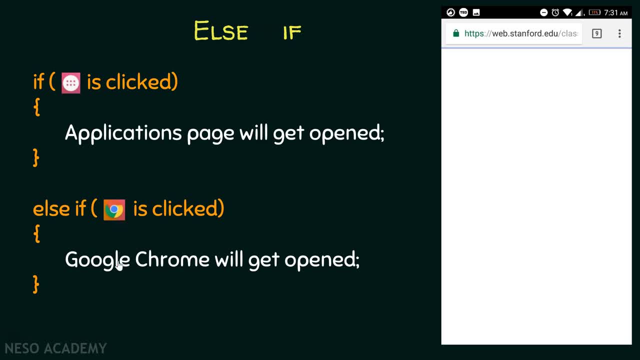 click on this button, that is chrome application button- then google chrome will get opened up. Therefore, whenever we have no dependency, we can use lsif, As this button clicking event is not dependent on this button clicking event, so we can use lsif. construct Right. 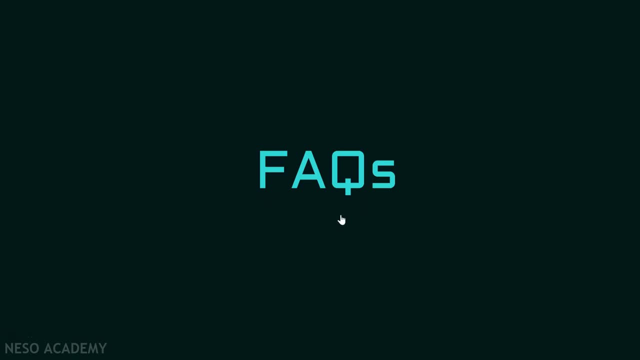 Now it's time for most frequently asked questions, That is, FAQs. Is it necessary to put the else part Now? somebody asked me this question: Is it really necessary to put the else part after the if part? The answer to this question is no. 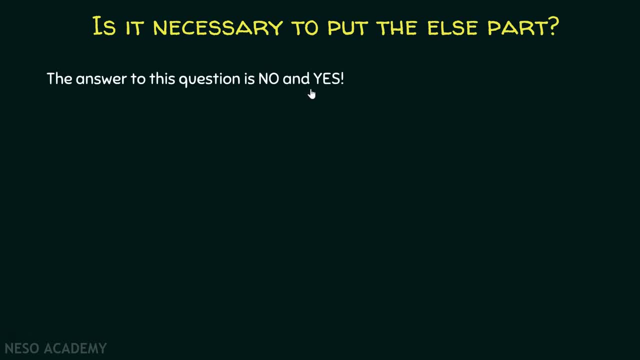 and yes, both at the same time. Let's try to understand this with the help of an example. Here you can see: I have a variable n and I have assigned it a value 4.. Apart from that, we are checking the condition. 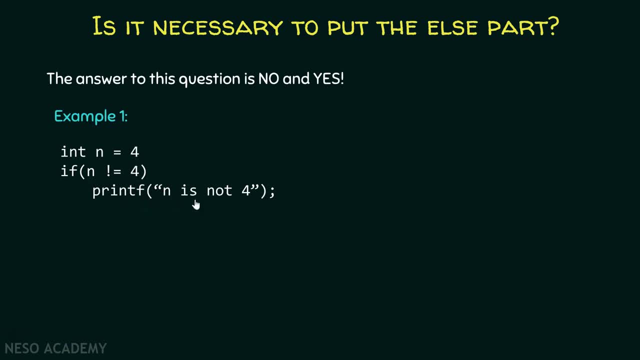 that if n is not equal to 4, then we can print: n is not 4.. Right, But here, as you can see, n is 4.. Therefore, this, if construct, will not get evaluated. One important point that you must have to note down. 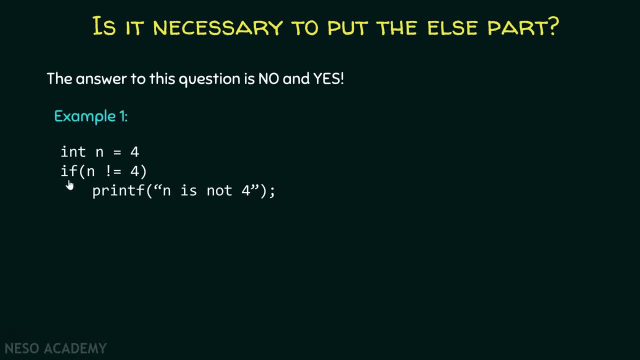 is that this printf function is actually the part of this if construct. Please note down Why, Whenever we have single statement written immediately after the if construct or else construct, then it is always considered to be the part of that if construct or else construct only. 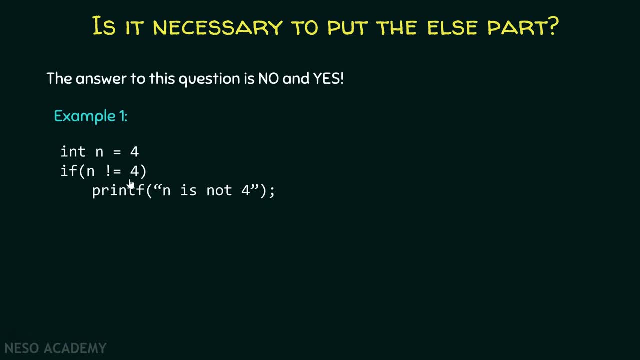 Okay, Here, immediately after this: if construct, you have a printf function which is just a single statement. Therefore, it is considered to be the part of this. if construct, only. Okay, This is the output of this particular program. The output is no output Right. 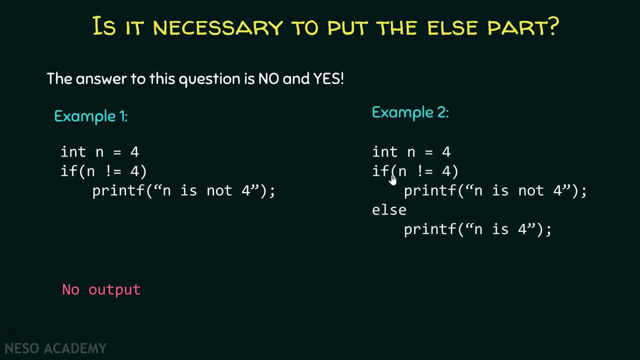 Let's consider one more example. Here there is very minimal difference between these two examples. This example is equivalent to the example one, But we have an else part as well. Here we are trying to print n is 4.. So the output is: n is 4.. 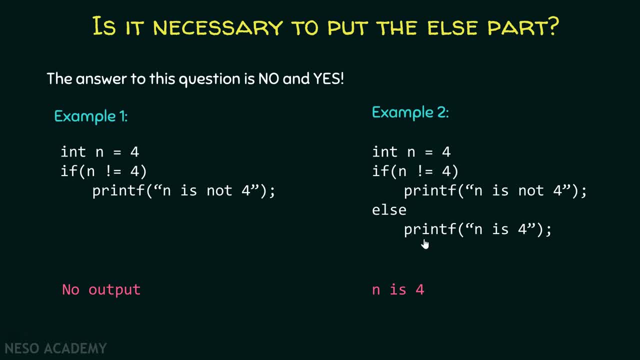 Because the condition itself is not satisfied. Therefore, the else part will get executed and it will print the statement: n is 4.. Right, As you can clearly see, it is not necessary to put else part if we didn't find the need to inform the user that n is 4.. 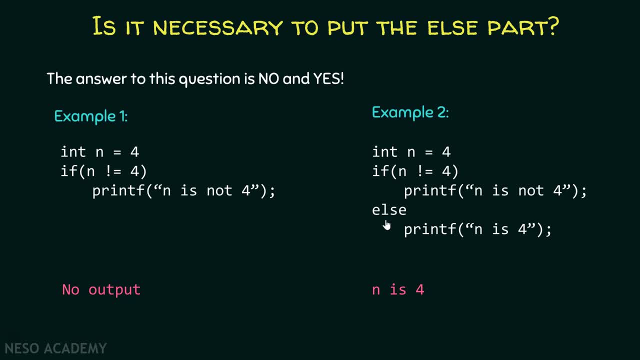 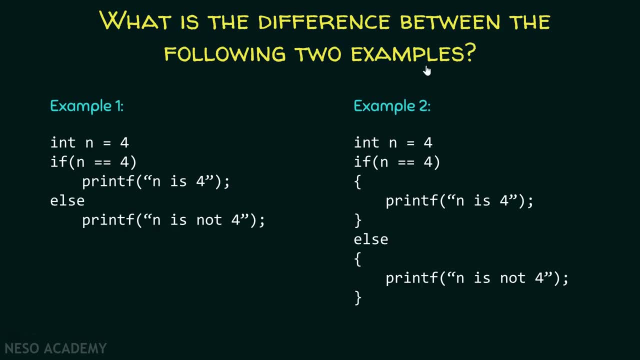 If we find the need to inform the user that n is 4, then we have to put the else part here Right? Let's consider one more question. What is the difference between the following two examples? In this example we are checking whether 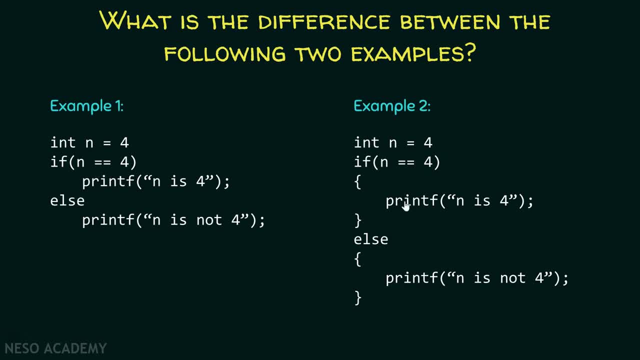 n is equal to 4 or not, And here also we are checking whether n is equal to 4 or not. Both are one and the same. If we talk about the difference between these two examples, then there is no difference. Please note down. 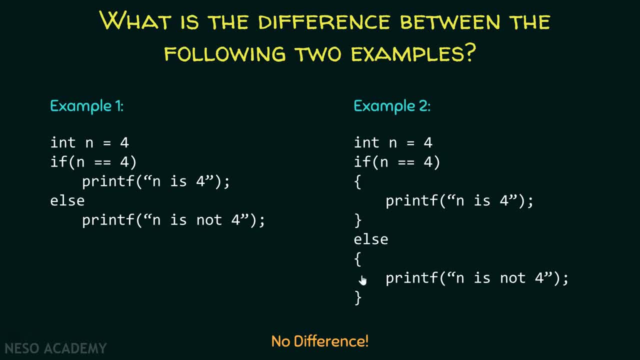 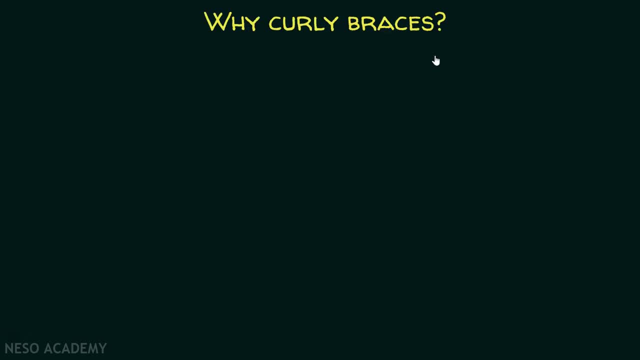 There is no difference between these two examples: Here you are putting curly braces and here you are not putting curly braces. Now you might ask me this question: then why curly braces? If it is really not necessary to put curly braces, then why do I need to put curly braces? 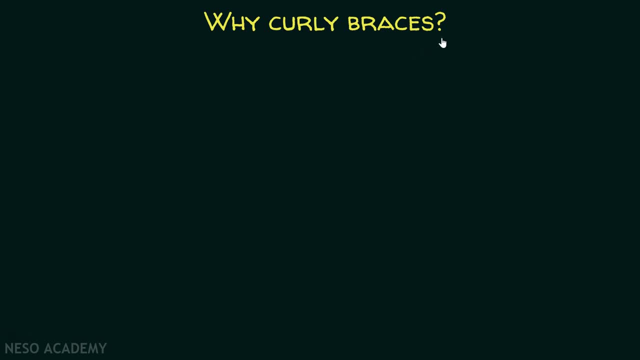 Let's consider one example Here. in this example, as you can clearly see, I have declared a variable n and I have assigned it a value 5.. After that, you can see there is an if construct and this printf is part of this example. 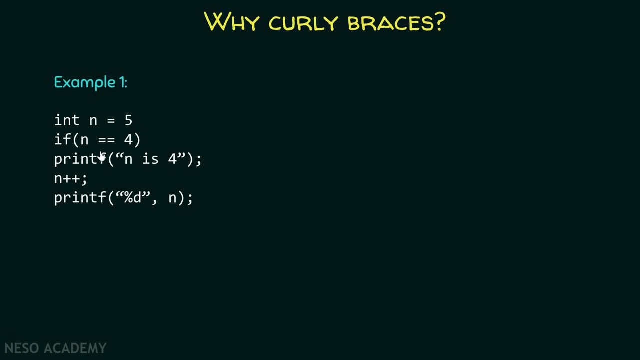 So I have declared a variable n, and this printf is part of this: if construct. As we know, whenever we have a statement written immediately after the if construct, then that statement is always the part of that if construct only. So this printf function is part of this: if construct only. 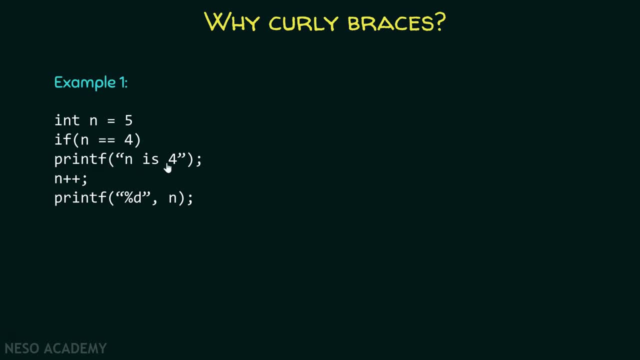 Now, as n is not equal to 4,, therefore, this printf function will not get evaluated, but n++ will get evaluated, Because n++ is not part of this, if construct Right, Therefore, the value of n is incremented to 6.. 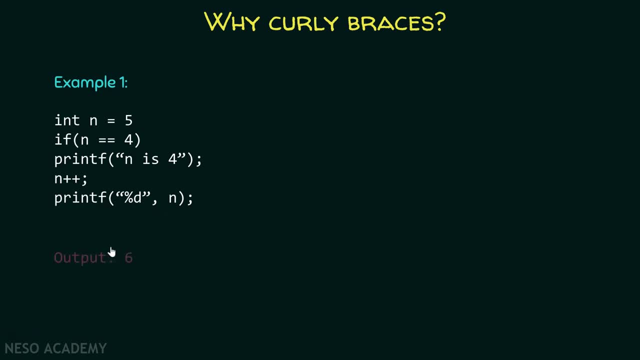 And after that the value will get printed. So the output is 6.. Right, Let's consider one more example Here. in this example, we are putting curly braces immediately after this, if construct, So that we would be able to include. 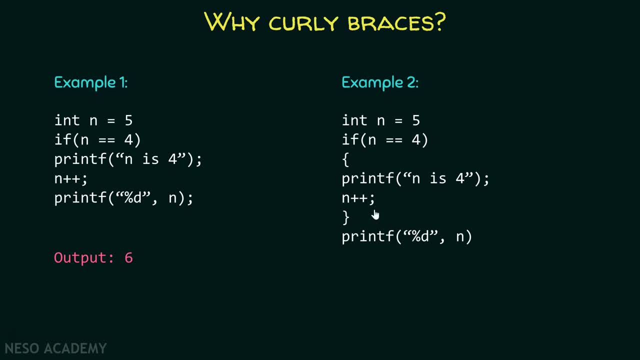 printf function as well as this n++. Now, if this condition is not satisfied, then the n++ will not get evaluated. Therefore, the value of n will not get incremented, As n is not equal to 4,. therefore, the value of n. 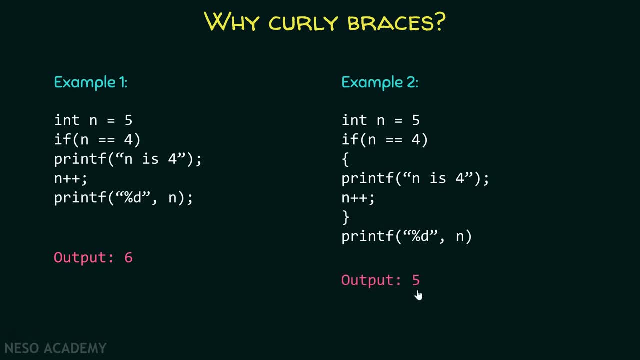 will not get incremented, And hence the output is 5.. Right, So we can clearly see that why it is necessary to put curly braces when we want to include two or more statements inside the if construct, If we just want to include a single statement immediately. 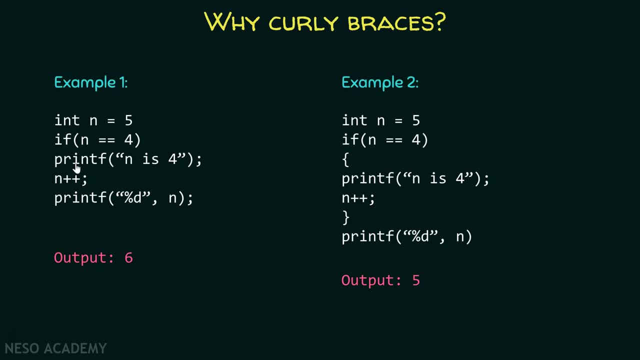 after the if construct, then there is no requirement of putting curly braces. But if we want to include more than one statement, then we have to put curly braces. That is what we need to understand about the curly braces. OK, OK, friends, this is it for now. Thank you for watching this lecture.